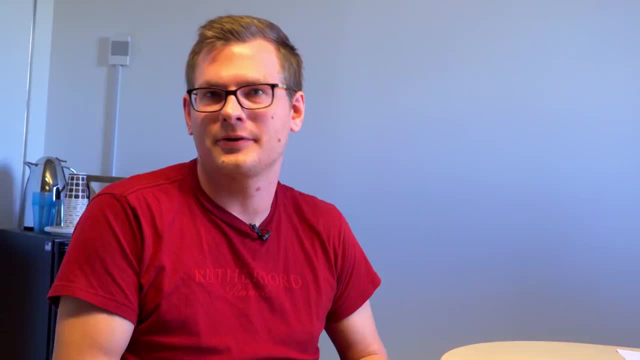 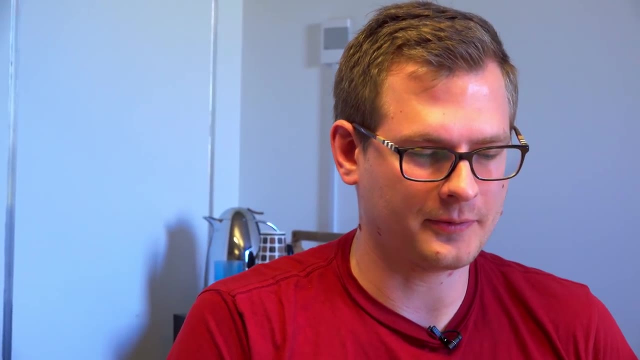 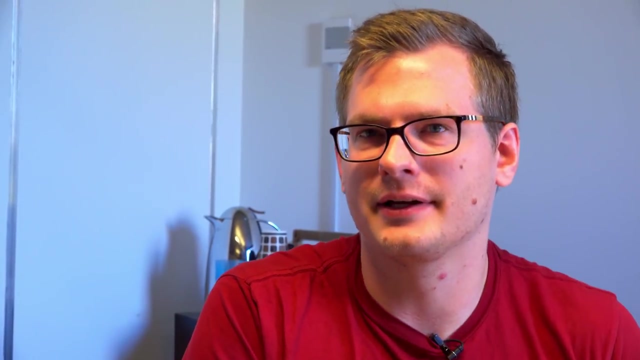 It can be used for any sort of task that you might want to do it for. It's a general purpose language, Lisp. It's been said that learning Lisp just helps you be a better programmer in general. It opens up a lot of different ways of thinking that are sort of locked away in languages like Java or C++ or what have you. 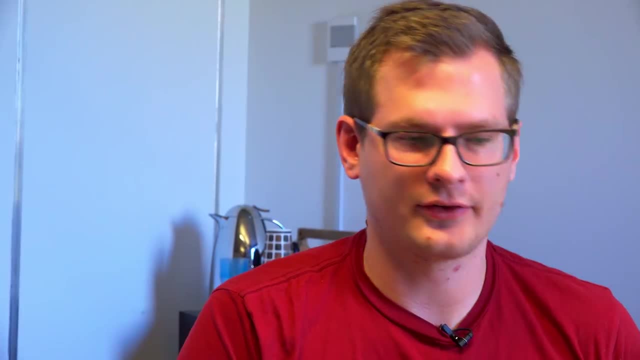 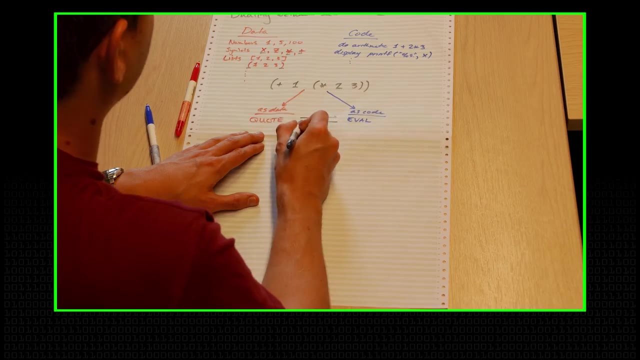 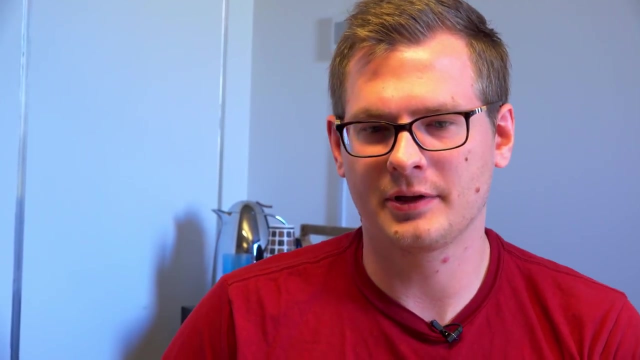 It has a few interesting ideas, such as this idea of homo-iconicity, where the language itself is written as a data structure that you can represent in that language. This idea of meta-programming, where not only are you programming in the language to solve a problem, but you can program the language itself. 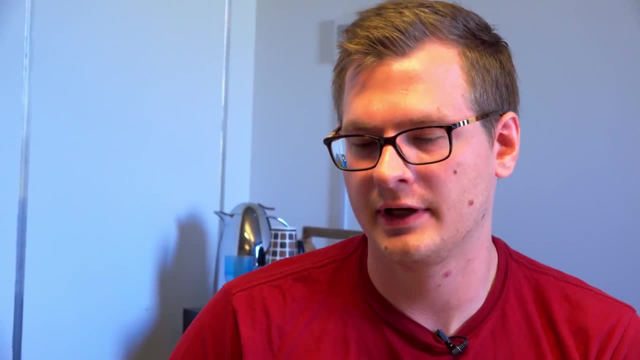 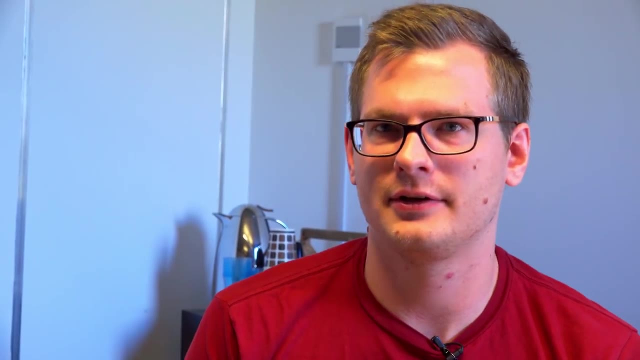 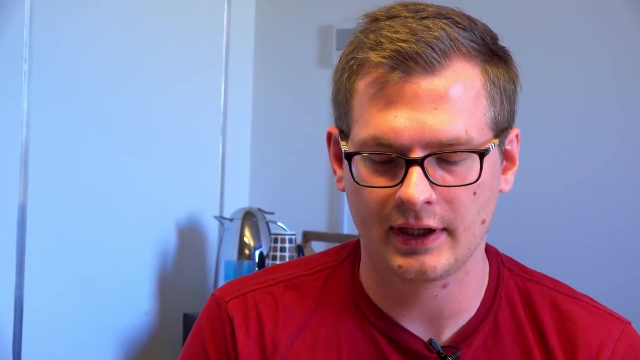 You can change the structure of the language itself to make it more suitable for a particular application, And even if it was just for learning those concepts, you become a better programmer in other languages. But nonetheless it still remains a language. Common Lisp in particular, remains a language that's very, very good at solving modern sort of real-world problems. 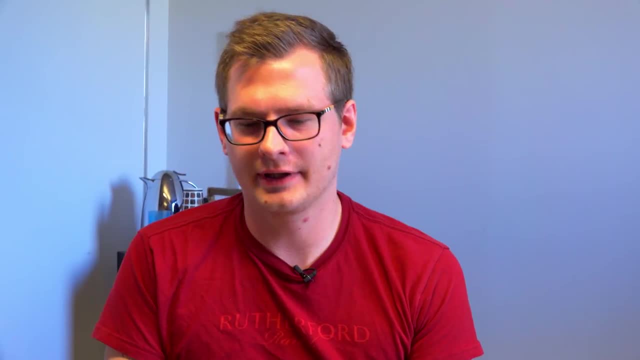 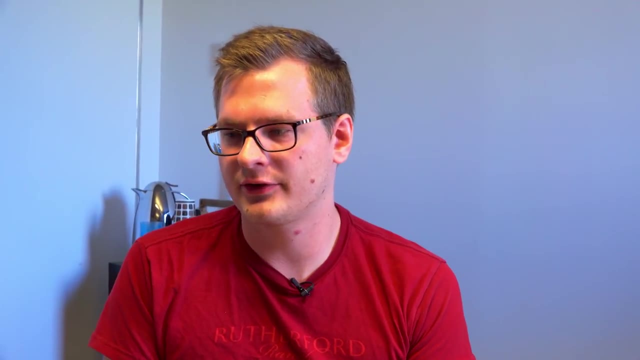 I actually would sort of draw analogy to physics, a little bit Like good ideas, ideas that are fundamentally good, are usually ones that stand the test of time. Now, computer science and computer programming is not a very old art, so to speak. 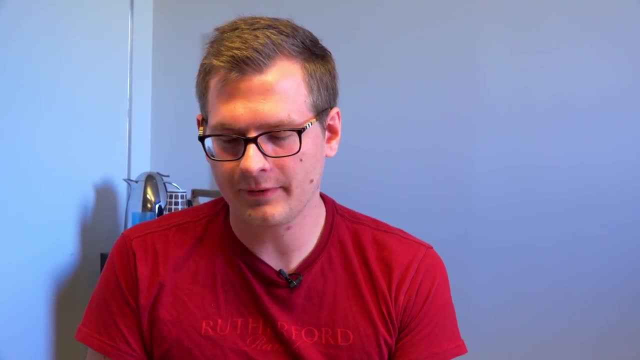 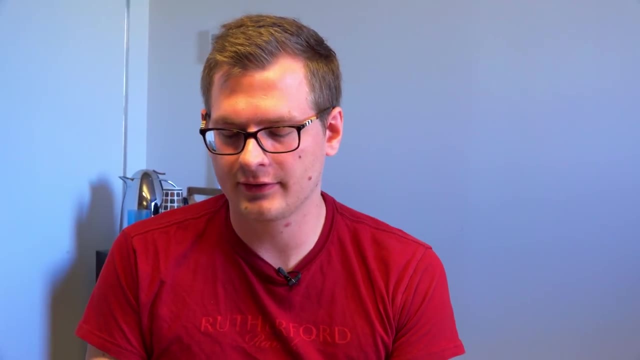 It's, you know, less than a century old. However, there are lots of theories, in physics for instance, that were sensible. They allowed you to make predictions. For example, the sun going around the Earth Seems reasonable, you see it. 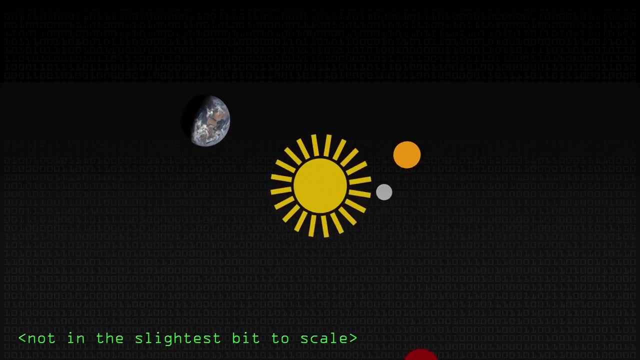 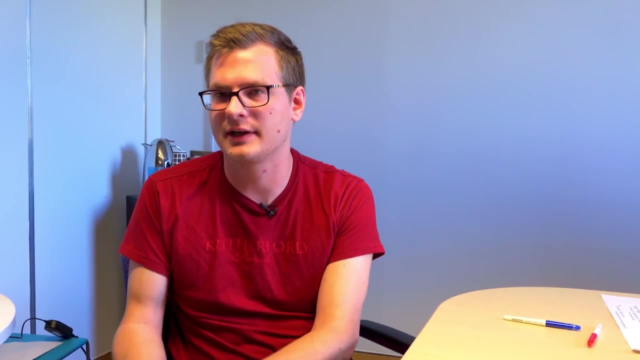 But there was a kernel of an idea later that the Earth goes around the Earth Or that the Earth goes around the sun, And that is a physical theory. that one turned out to be true but also stands the test of time. There are good ideas in it that are fundamentally good. 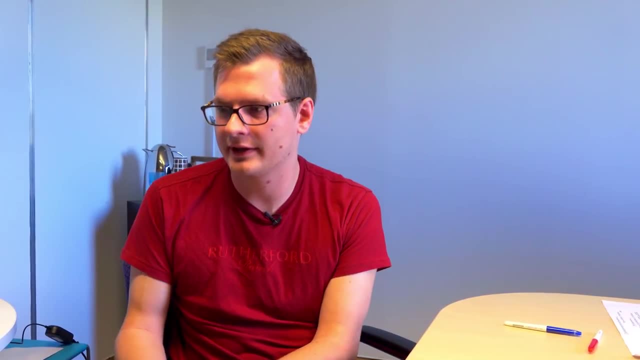 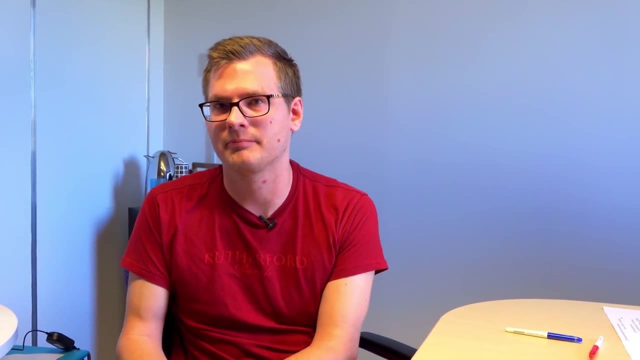 And so I think that just the fact that Lisp is started in the 1950s and still has something, still has some kernel of an idea, that's good, I think, makes it worth learning, even if it's not used day to day. 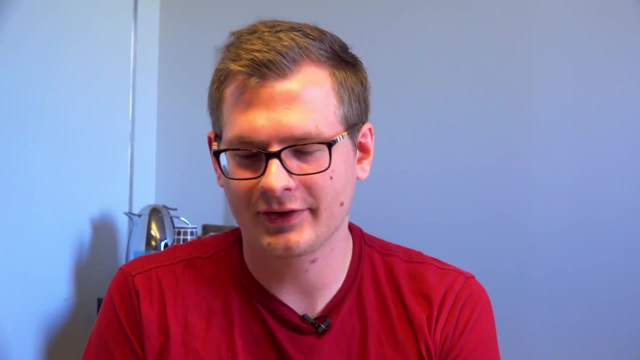 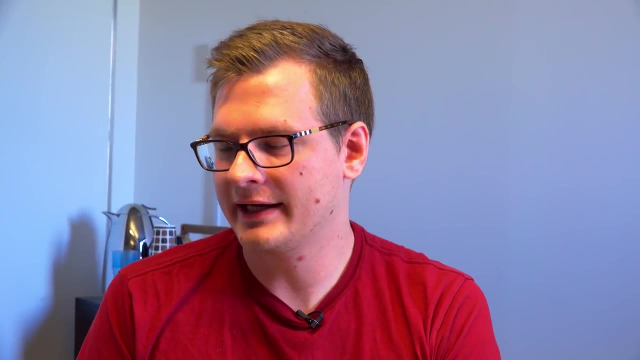 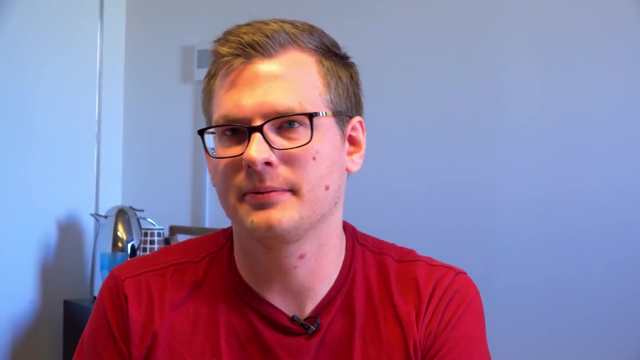 You do use it day to day, don't you? Yes, yes, Yeah. So, Lisp, even still going back to this kernel of an idea, is good. It's good at building a language that I want, So I can't think of anything that's better than using a programming language that allows me to build the language that I need to express my problem. 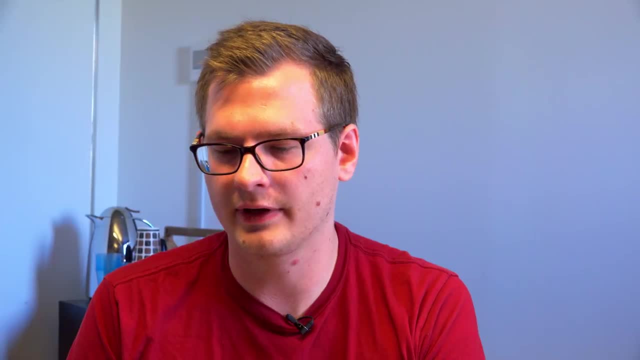 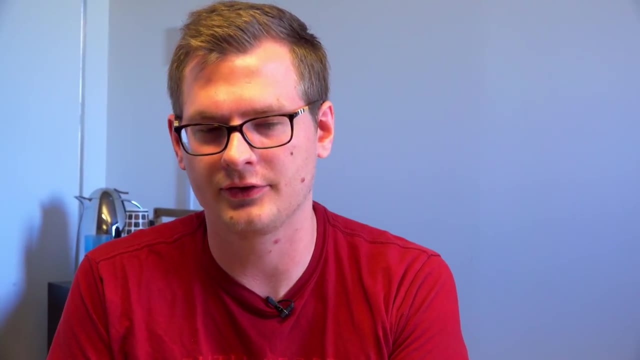 The stuff that I work on day to day is quantum computing, where there isn't a lot of literature on how to wrangle the problems that come up in quantum computing. Quantum computing uses quantum mechanics, which is a very, very different mathematical language than just addition of numbers, for instance. 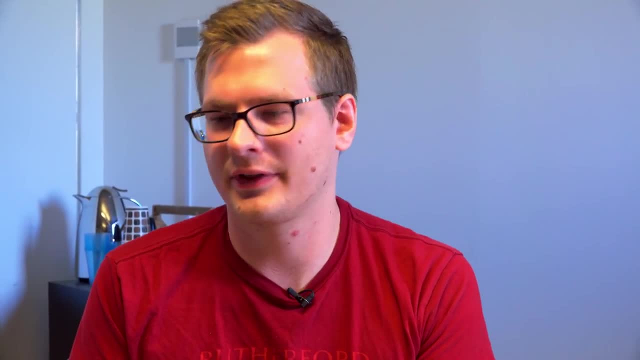 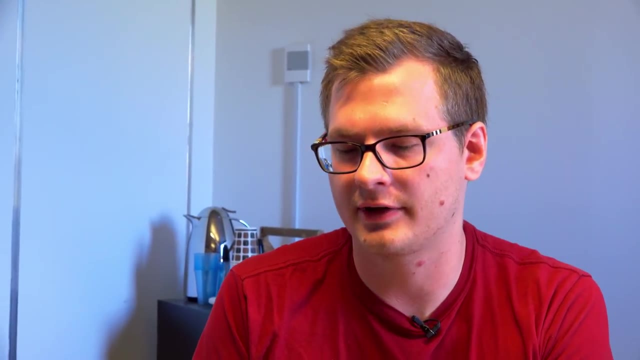 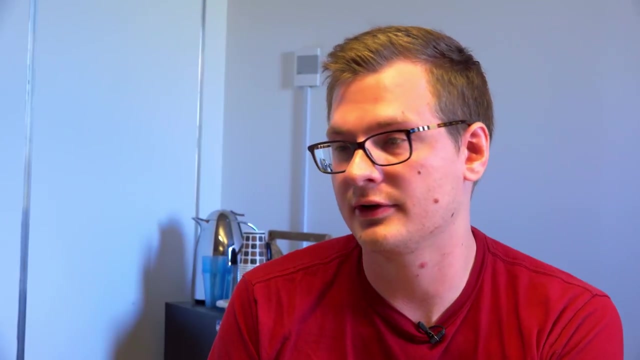 It is a very strange world where things have all different types of rules, So modern programming languages don't support expressing these constructs in a very fluid way. So often I need to build my own sort of language in order to express solutions to problems that I'm having. 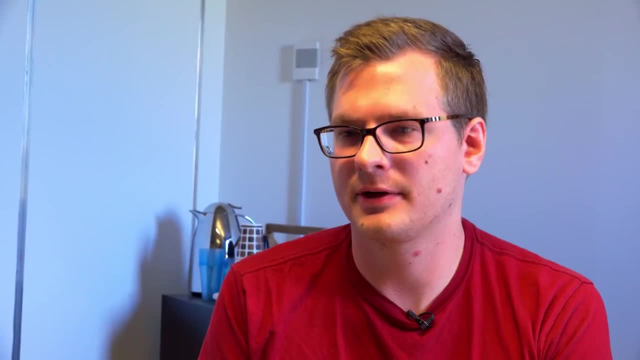 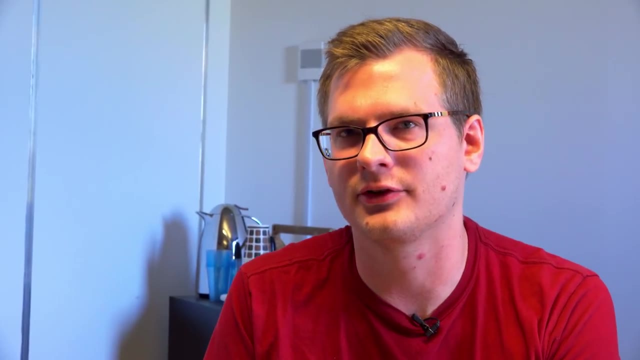 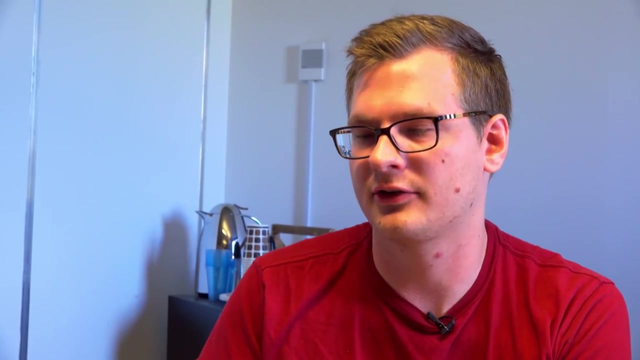 Now you can do this in a language like C++ or Java. You can build your own parser, You can build your own compiler, You can build all of the things you need to just be able to write solutions to problems. But in Lisp it allows you to grow the language ever so slightly in a very easy way, so that in Lisp directly I can express these new constructs. 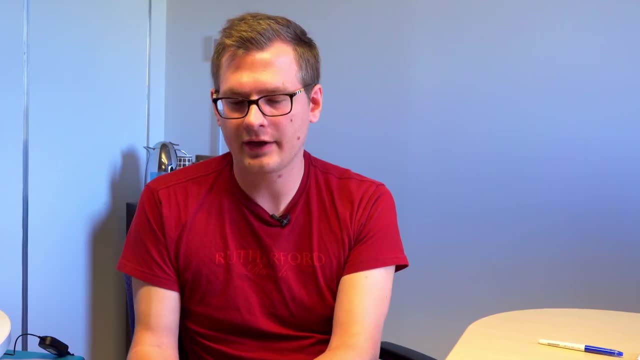 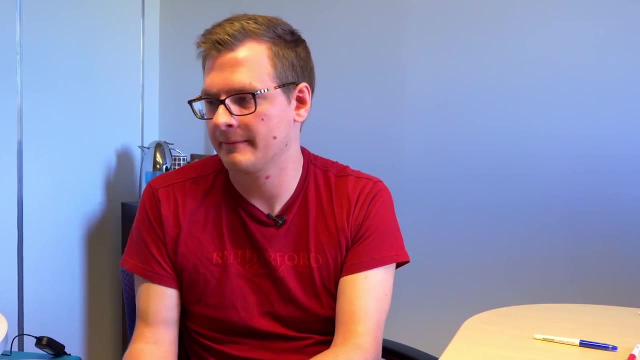 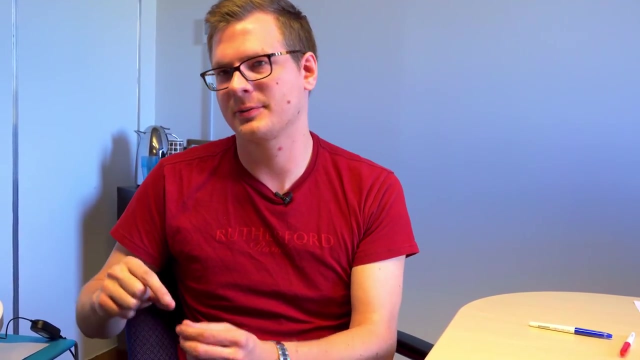 And it's very helpful for these types of new domains. We're actually extending the syntax of the language. So one example that I like to bring up is back in the days of programming assembly, if you wanted to do something like a for loop, you wrote down the structure where you have, like this explicit jump statement: 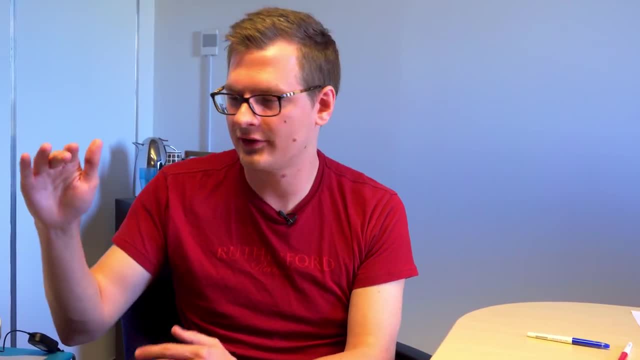 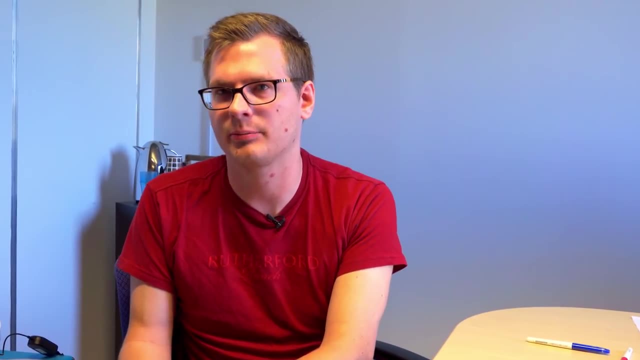 You say: and then you have a separate counter, You write it somewhere And it's all just a bunch of lines of assembly, Nowhere in the assembly code. are you actually saying like for i from 1 to 10, or something like that? 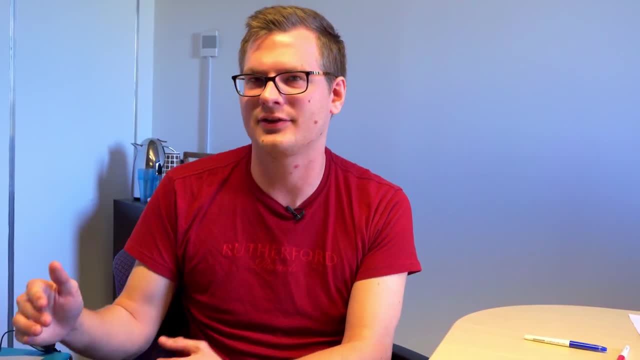 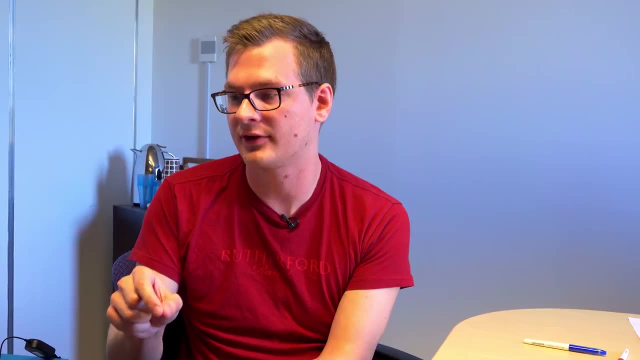 But you know, the concept is there. You know, as the programmer, what you mean by these instructions is a for loop. What Lisp does is allow you to take that idea of a for loop and actually syntactically be able to write a for loop. 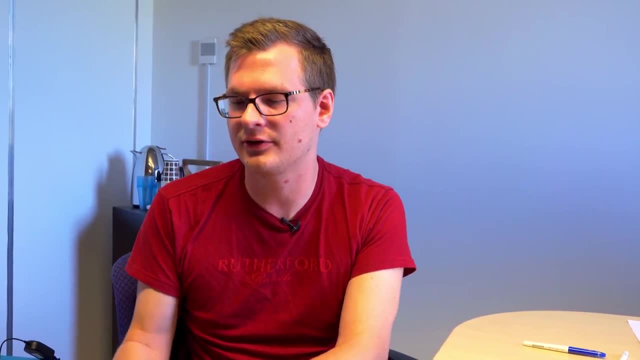 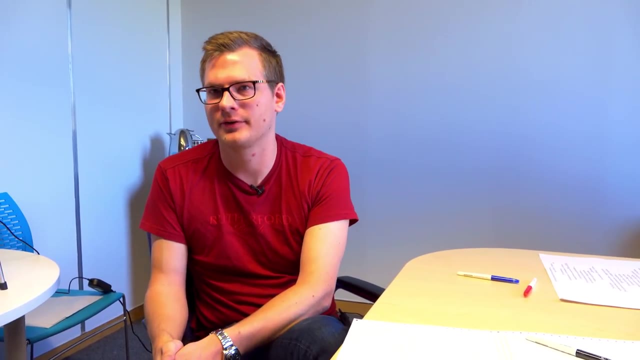 So it's not just a library of functions, It's actually new syntax and new functionality in the language. But it all does come down to assembler in the end, doesn't it? Yes, Absolutely Yeah, It all gets compiled to assembly in the end. 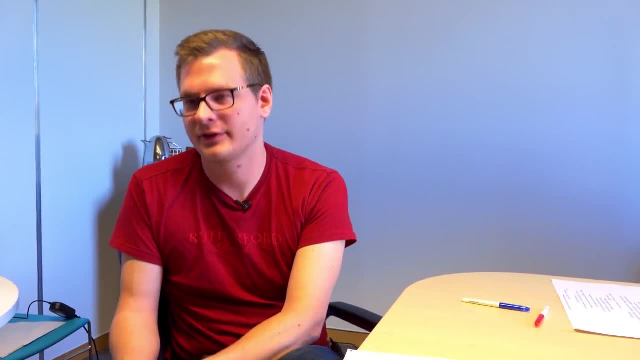 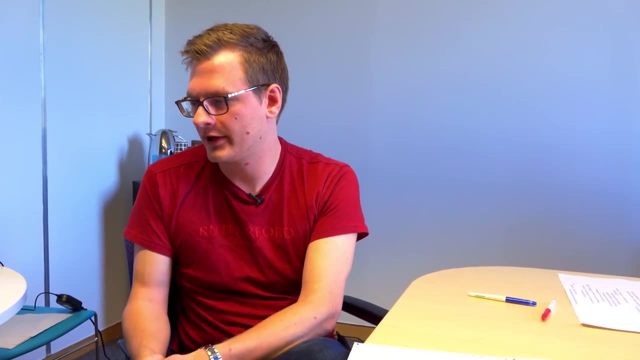 So this is a way of organizing your thoughts as a programmer, Correct? Yes, Yes, That's, I think. ultimately, what it's optimizing for is allowing you, the programmer, to organize your thoughts, And most of the time in programming is spent thinking. 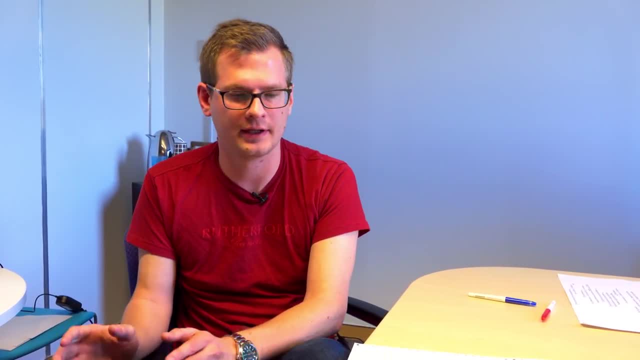 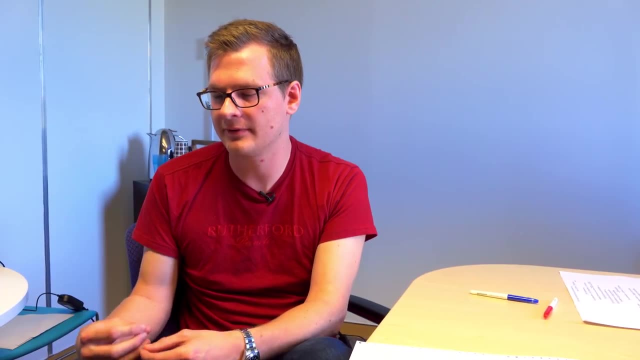 And so that's the process that I want to optimize in programming, Not necessarily the efficiency of the program, although you can do that And other things- It's being able to even get the solution to the problem out on paper, on the web.